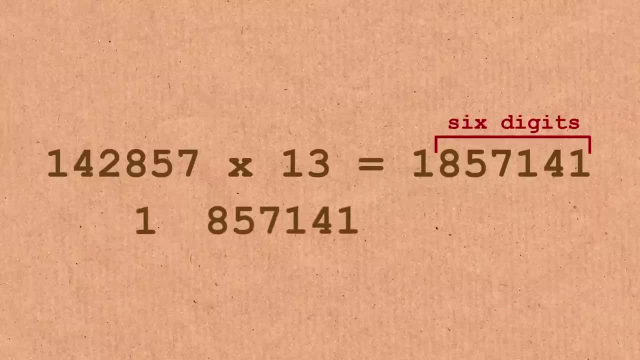 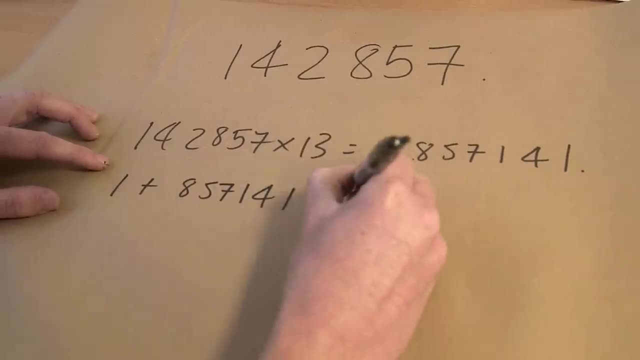 I'm going to take the last six of these and I'm going to add it to the first one, So that's 1 plus 8, 5, 7, 1, 4, 1.. Now I can do that. That is 8, 5, 7, 1, 4, 2.. 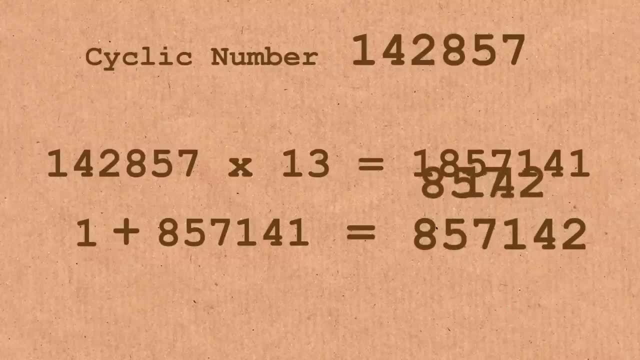 Which, if you look carefully, is a permutation of this guy. So it's 1, 4,, 2, 8, 5, 7.. Give me another number, Brady. Give me another number: 112.. Right, 112.. Very good. 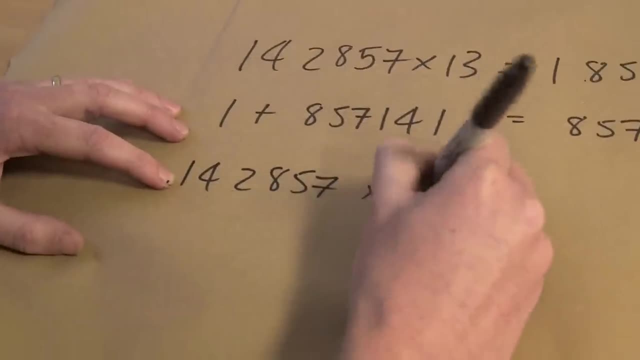 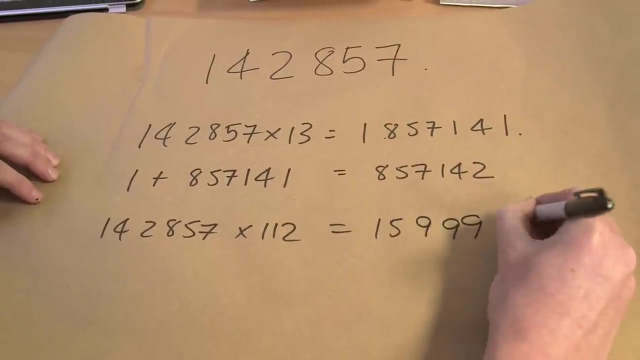 So 1,, 4,, 2,, 8,, 5,, 7 times 112.. 112 equals right. Let's do it. Okay, I noticed something about 112.. You're a pain for choosing 112, but we see something else. 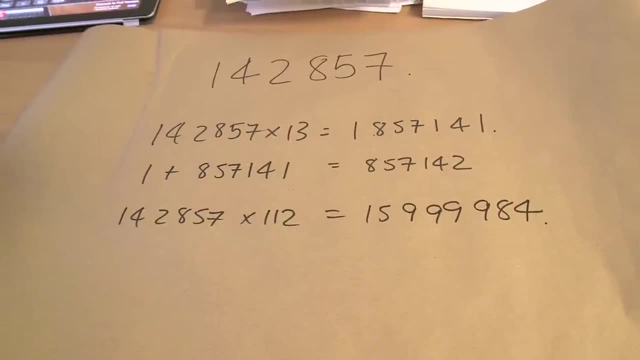 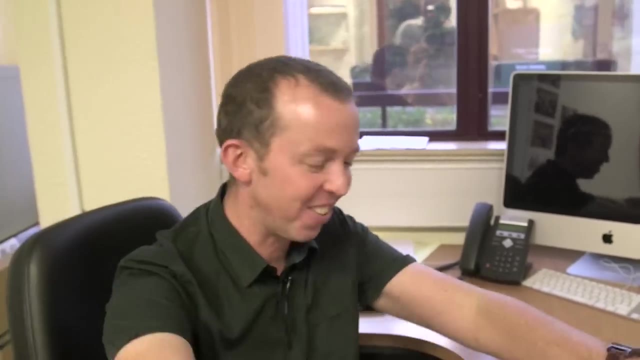 Okay, 112,, I think, must be a multiple of 7.. In fact, it is Right. You ruined it with it. What The multiples of 7 bring us. Multiples of 7 are the only ones. If they do something else, they do something else. 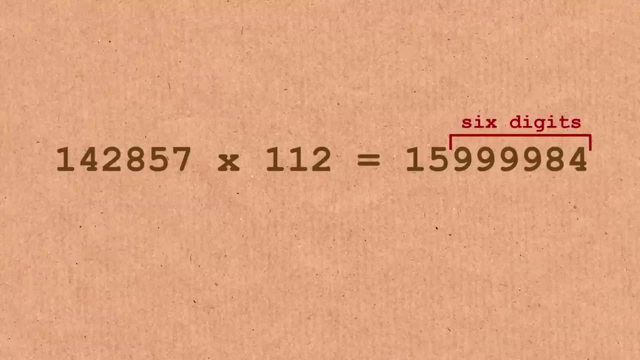 Let's run with it. Let's run with it, Okay. multiples of 7.. I will do it. We'll take the last six. Okay, 15 plus 999984 equals 9,, 9,, 9,, 9,, 9,, 9.. 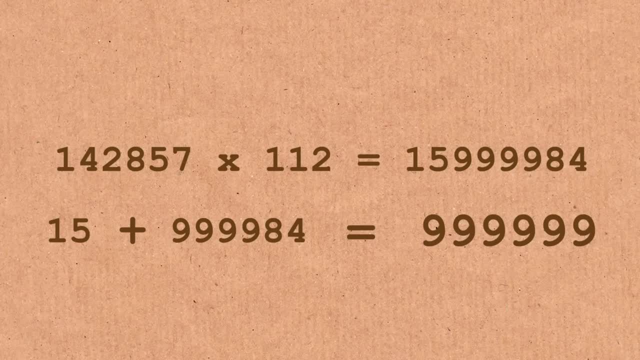 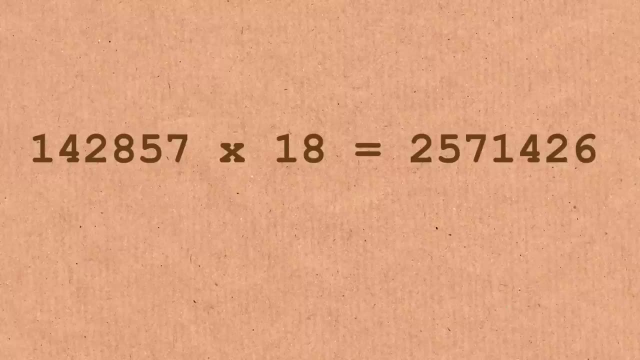 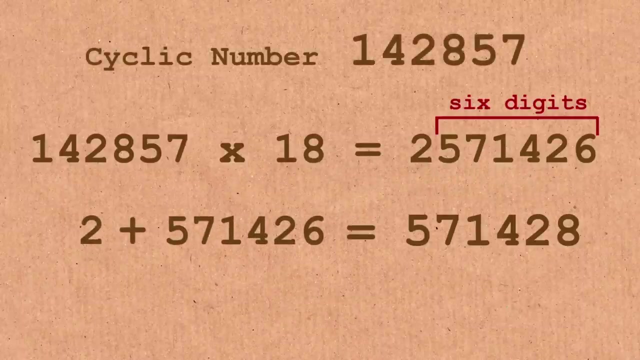 Okay, Give it, we'll do one more. okay, 18. 18.. Okay, not a multiple of 7.. Thank you, 2,571,426.. Do the same thing. Take the last six And I get 5, 7,, 1, 4,, 2, 8,, which is 1, 4, 2, 8,, 5, 7.. 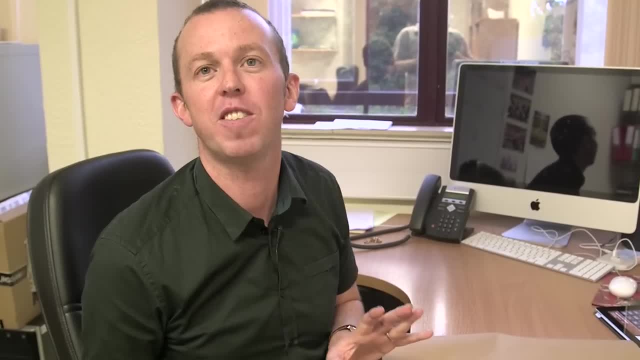 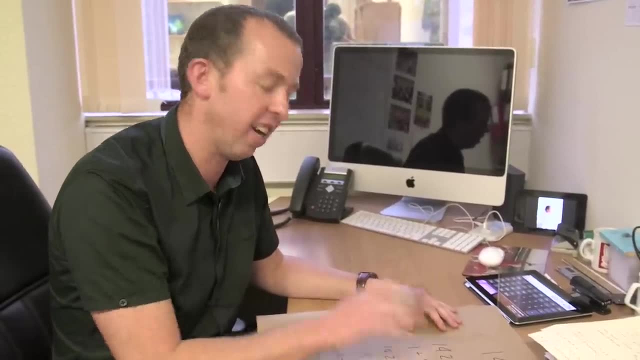 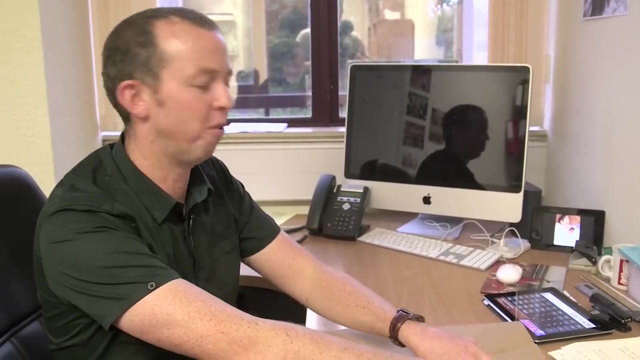 If I take anything that's not a multiple of 7, anything that's not a multiple of 7, and I multiply this number by it, and then I do this procedure of sort of taking the last six and adding the previous one or the other ones, I always get a permutation of 1, 4, 2, 8, 5, 7.. 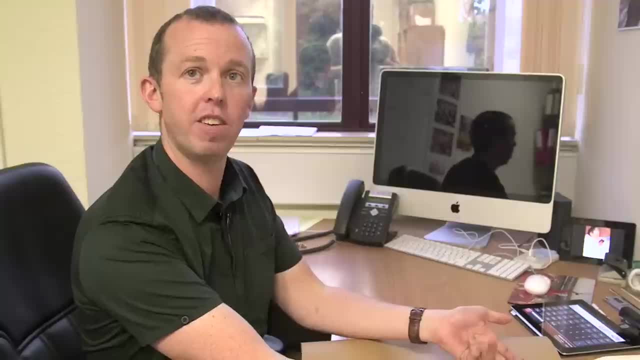 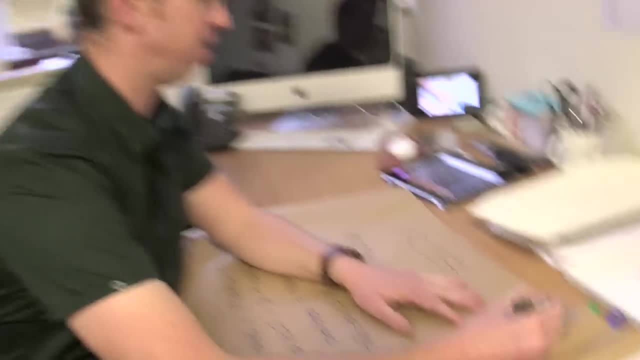 In particular, if I take the numbers 1 to 6, the six digits here, and I multiply this by them, I will always get a permutation of 1,, 5,, 7.. So for example, obviously if I multiply it by 1, I get 1,, 4,, 2,, 8,, 5,, 7.. 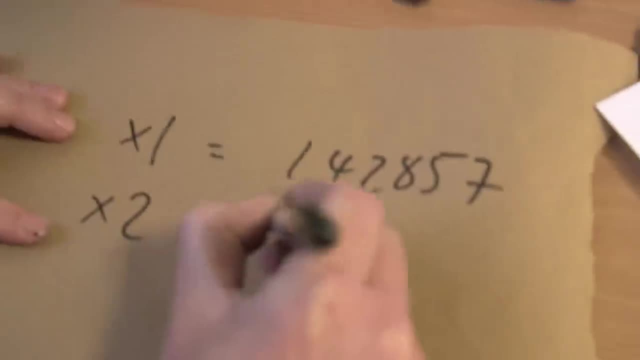 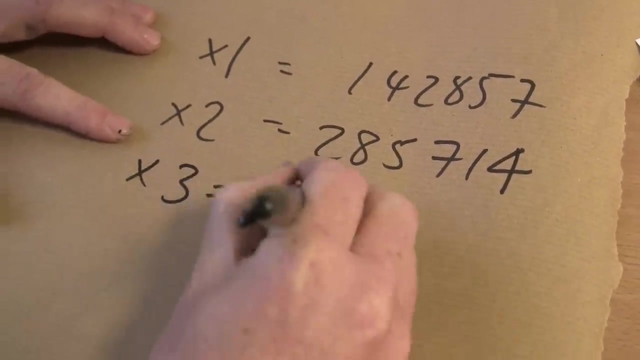 That's trivial. If I multiply it by 2, I get 2,, 8,, 5,, 7,, 1,, 4,, which again is a permutation. multiply it by 3, I get 4,, 2,, 8,, 5,, 7,, 1, and so on and so forth. 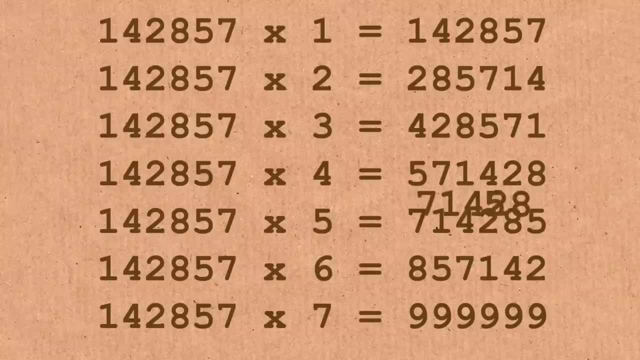 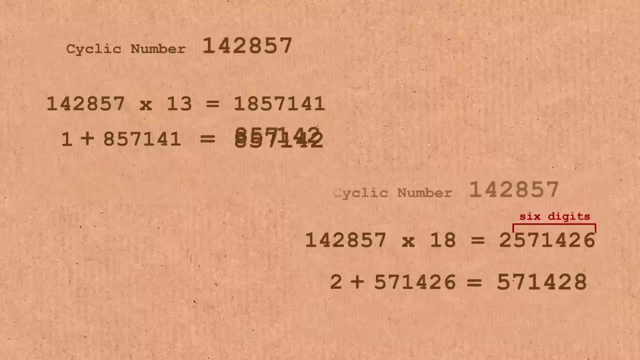 And I can keep doing this. And if you go above 7, then you need to do this business of sort of taking the last six and then adding it, But you'll always get this cyclic structure. This is an example of a cyclic number, in fact. 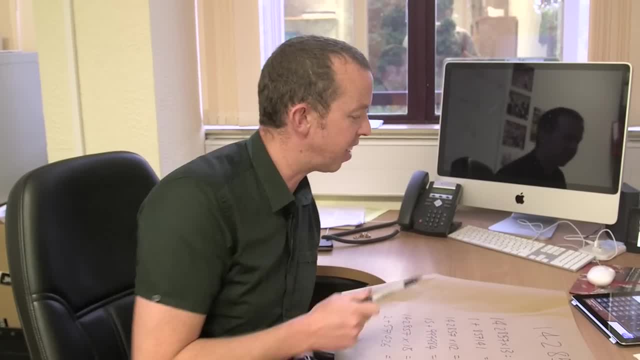 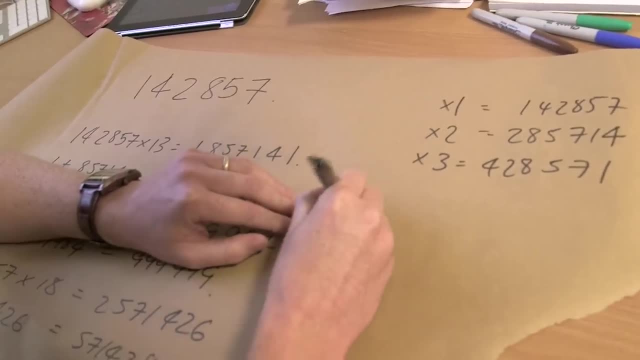 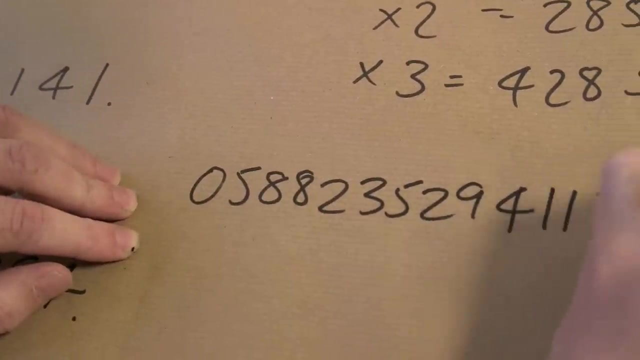 A common Right. Not particularly Okay. So this is the only one that doesn't begin in 0.. The next one, actually after this one, is 0, 5, 8, 8, 2, 3, 5, 2, 9, 4, 1, 1, 7, 6, 4, 7.. 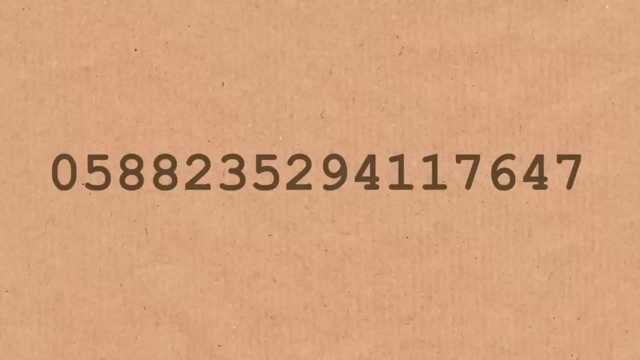 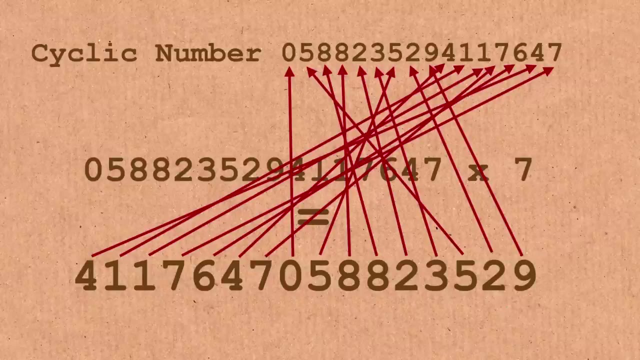 This is another cyclic number. Okay, This has got 16 digits. You play the same game. You can take In this. now you would multiply it between. What's important is the fact it's got 16 digits, So if you do multiples of 17.. 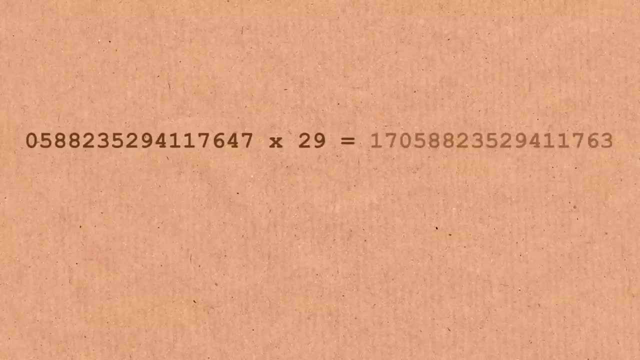 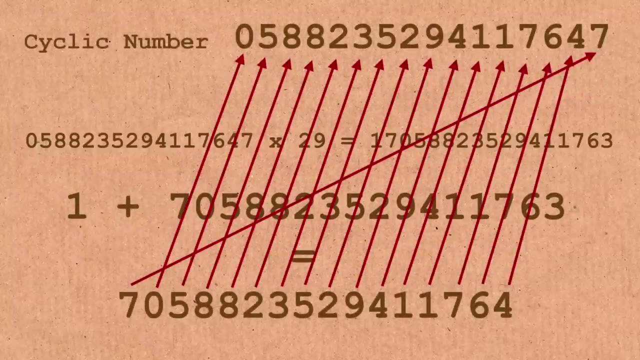 It goes wrong. but if you do 1 to 16, you'll get a permutation of it, and then you can play this game as well, but with 16 rather than 6 digits. So here's the other weird thing about it. 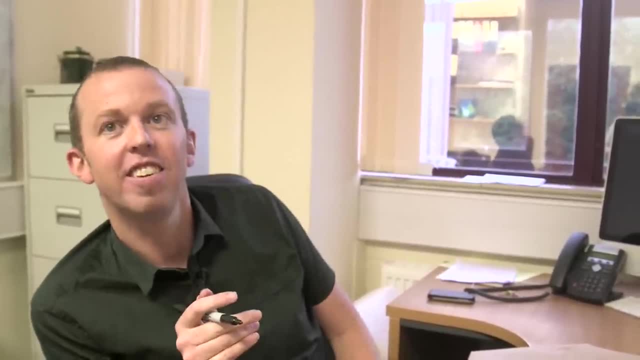 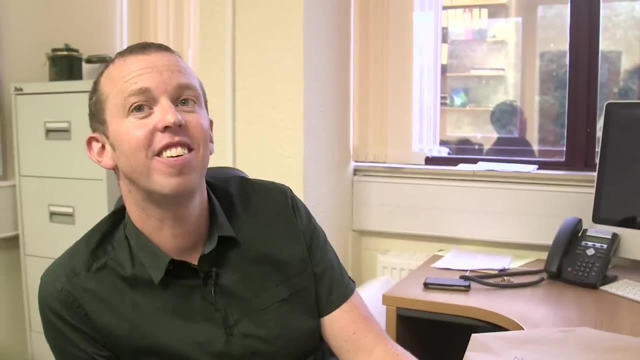 If you multiply it by any multiple of 7, you always get these all the 9s. If I multiply this guy, this has got 16 digits. If I multiply this by 17,, I'll get all the 9s. 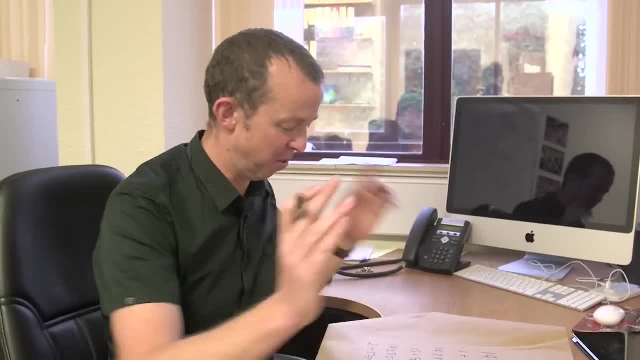 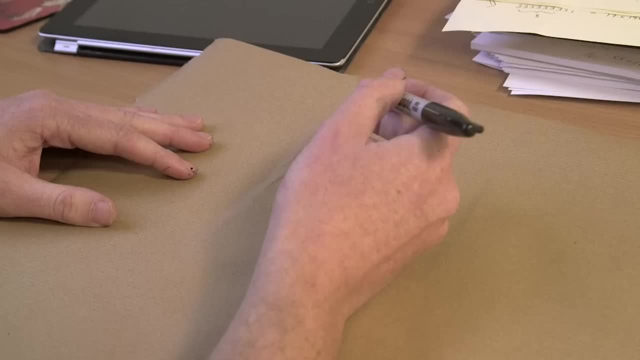 Why does it work? Okay, Let's see why it works. I'm going to need more paper. No, Okay. Well, the important thing about this is that. Okay. Well, the important thing about that number- that 1,, 4,, 2,, 8,, 5,, 7, is it appears in the decimalization of a 7th. okay, 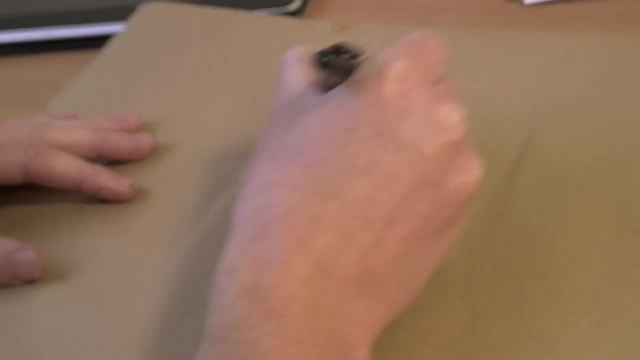 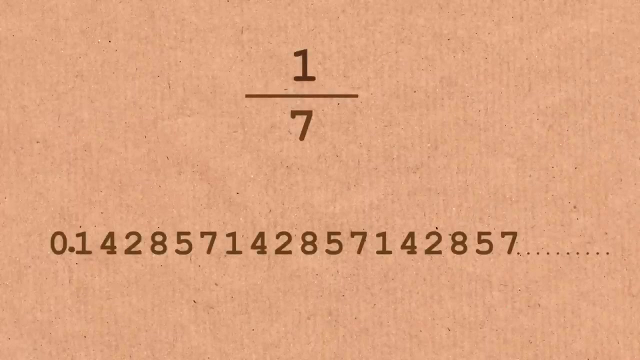 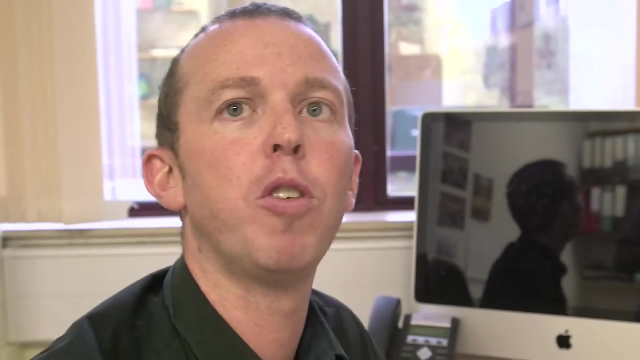 If I take a 7th right, then a 7th is equal to 0.142857142857,. do-da-da-da and so on, Keeps repeating, And this is critical. Why is this critical? Well, now think what happens when I multiply this by 10.. 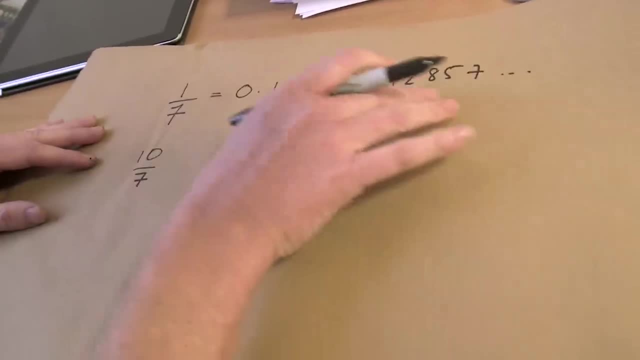 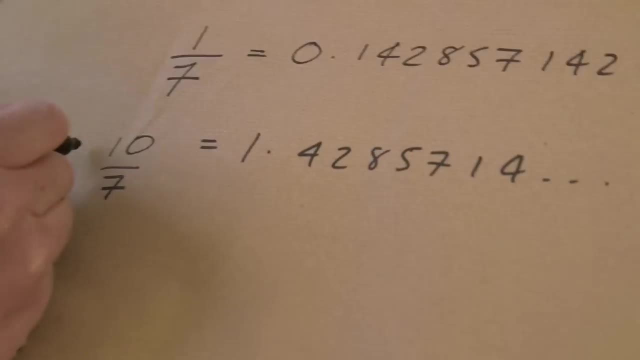 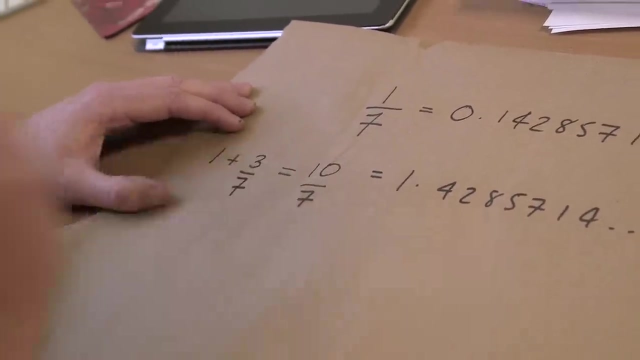 I multiply it by 10.. 10 7ths, I multiply it by 10,. all these numbers just shift along. 1, right And now. But what do you know about this? This is just 10. 7ths is 1 plus 3 7ths right. 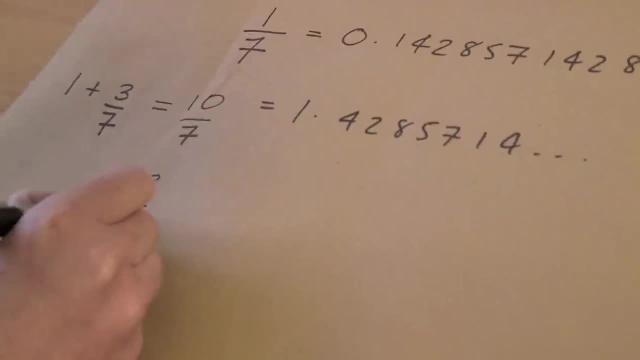 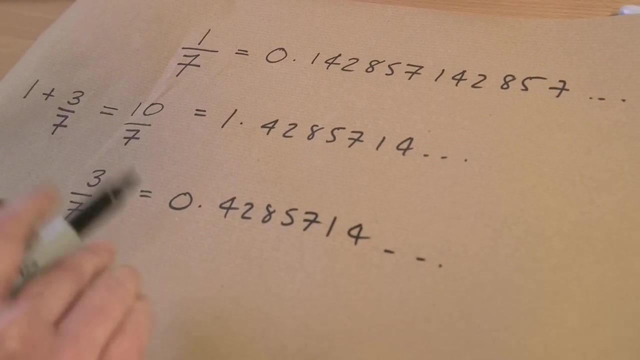 Okay, So from this you can infer that 3 7ths is equal to 0.4285714,. do-da-da-da-da. And the point is is you can see that all, So I multiply it by 10, just shifted everything along 1, okay. 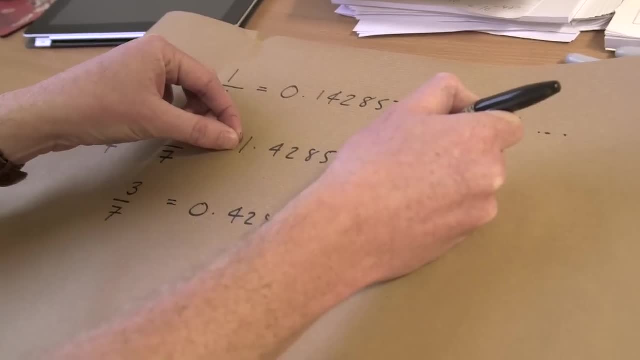 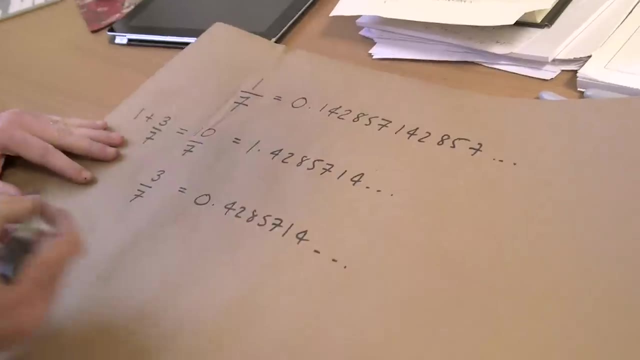 And then we pull off this original 1, but it got replaced by another 1 and getting shifted along, And then you're left with a permutation. It works perfectly And it keeps working. Now we can do the next one, say: 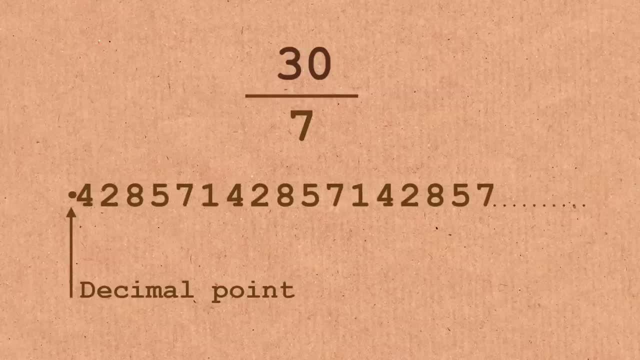 Multiply it by 10 again. So I do multiply it by 10, do 30 7ths and I get again. I just shift everything, just get shifted along by 1.. But this I know is 4 plus 2 7ths. 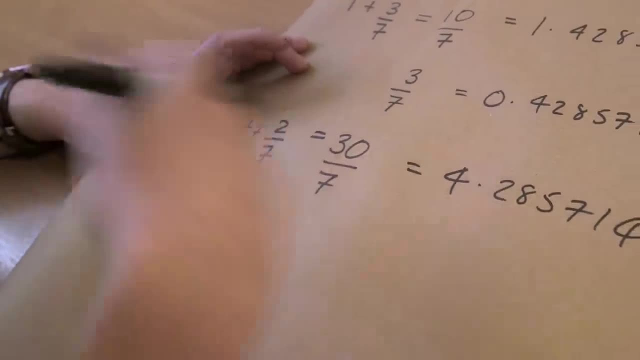 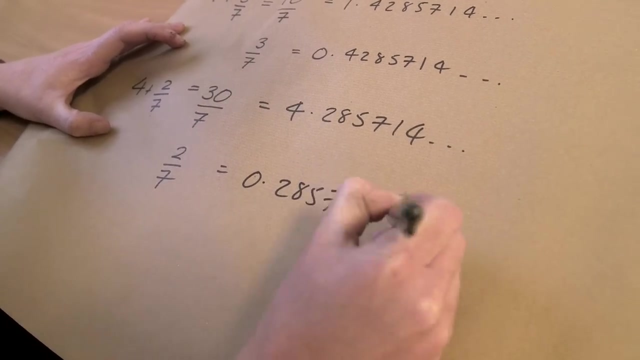 So I multiply it by 10.. I multiply it by 10.. I multiply it by 10.. So I get rid of the 4s and I conclude that 2 7ths is just 0.285714.. And again it was just. everything got shifted by 1.. 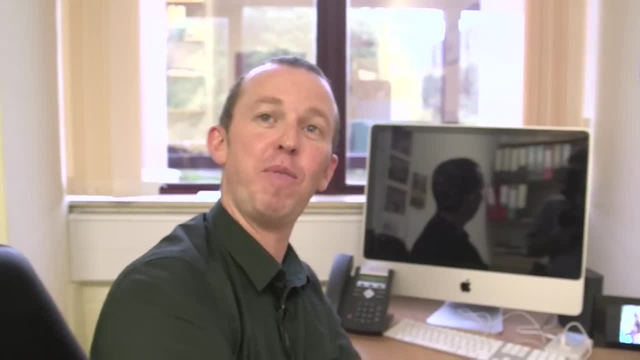 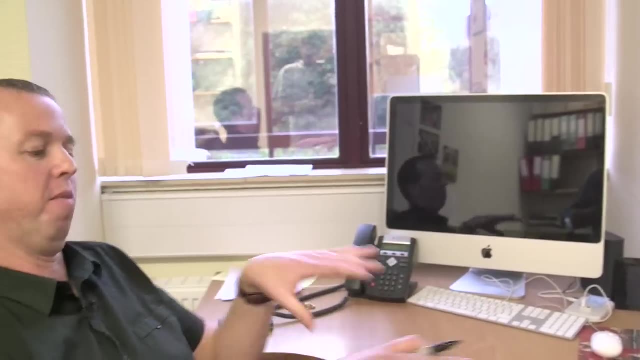 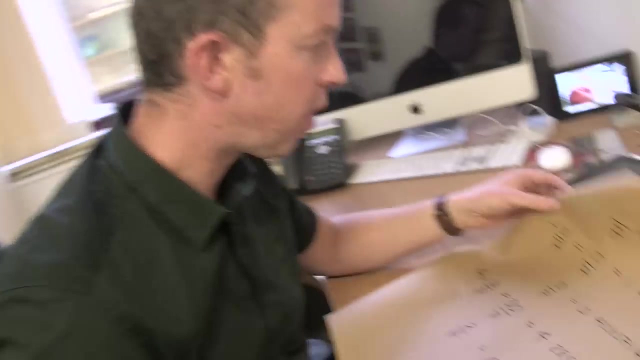 But because it was the stuff that you removed that replaces it. you just end up with permutations, And that's why it works. That's essentially the essence of why it works, And actually from this structure you can see why, What the structure of all these cyclic numbers has to be. 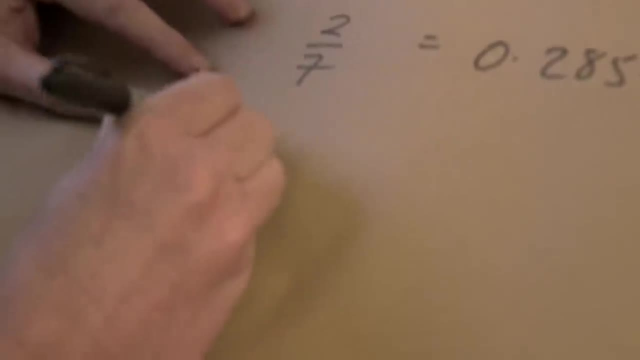 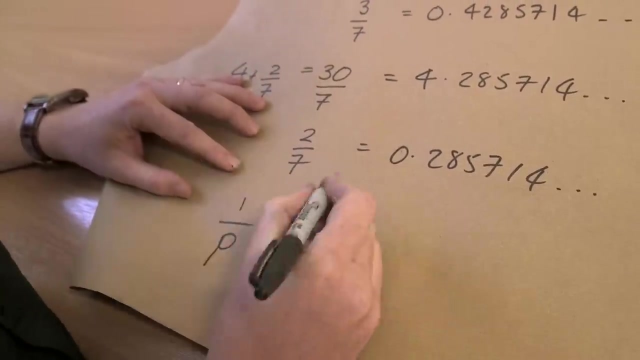 So you take A prime number, you take its reciprocal 1 over a prime. OK, It doesn't work for all prime numbers, but for some prime numbers it does. Actually, we'll come back to that in a minute. 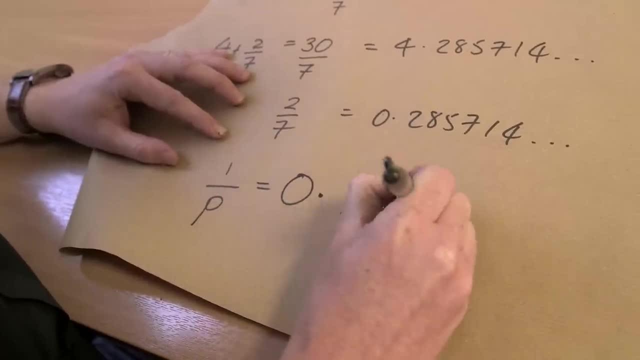 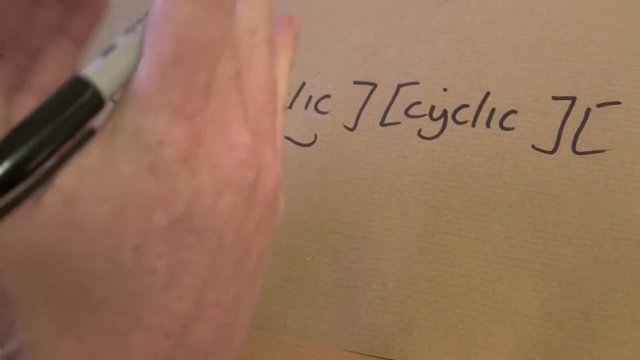 But you'll get something: 0 times your cyclic number, And your cyclic number gets repeated. OK, This is a p minus 1, a number of length, p minus 1.. So here it was a 7th, and these blocks had a length of 6, OK. 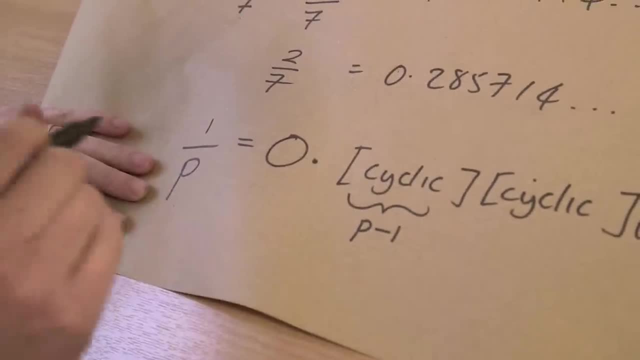 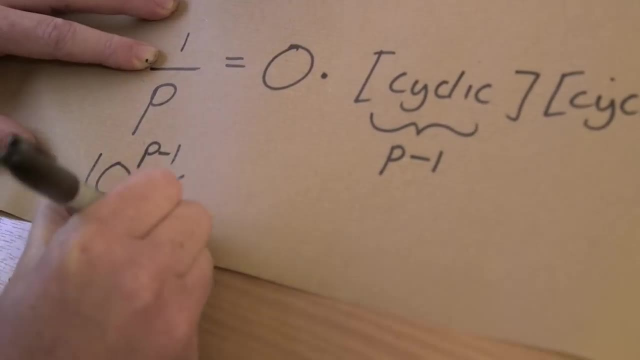 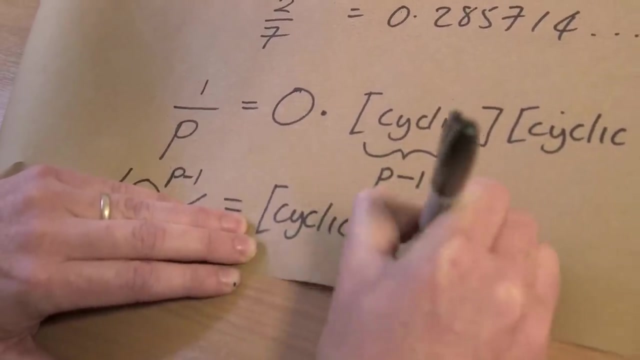 So if I multiply this, So if I multiply this by 10 to the power p minus 1, in this case by 10 to the 6th, I get 10 to the p minus 1. over p is equal to well, my cyclic number point, my cyclic 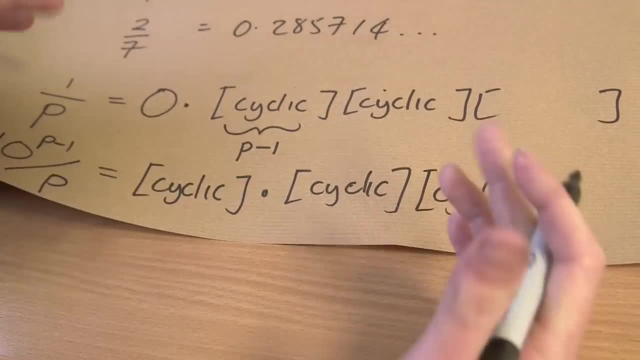 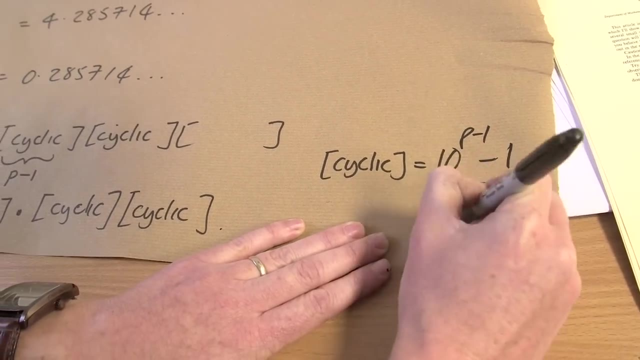 number. So you get all the. You get the same thing. Now you take these two away from one another and you conclude that your cyclic number is equal to 10, to the p minus 1, minus 1, over p, And this is where those knives come in. 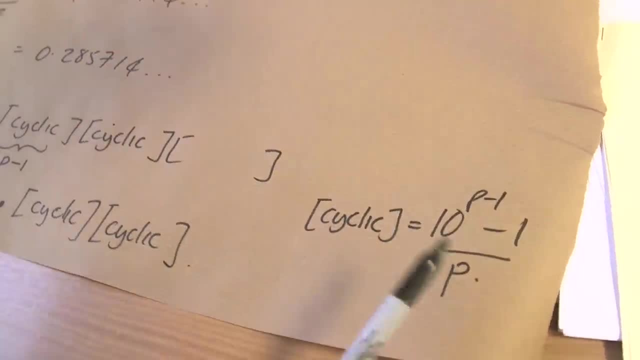 OK, This is where the 9s appear. OK, Because if I multiply this by p, the prime number, which in this case was 7, or any multiple of 7,, I get something that's related to the 9s, right. 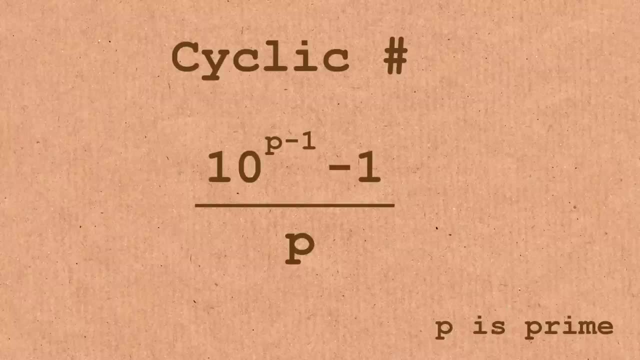 Because it's 10 to the sum power minus 1, which is going to be all the 9s, Right? So that's why it works. All the cyclic numbers have this form. Not all prime numbers will give a cyclic number when you construct this guy. 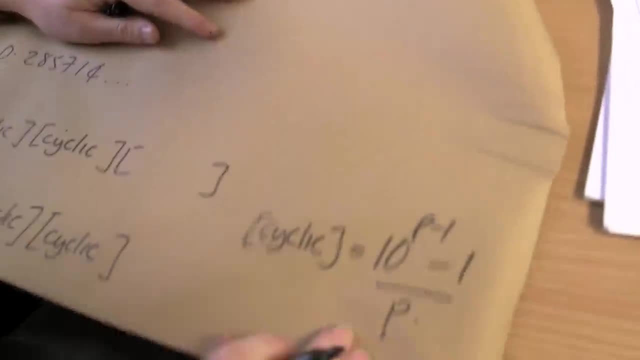 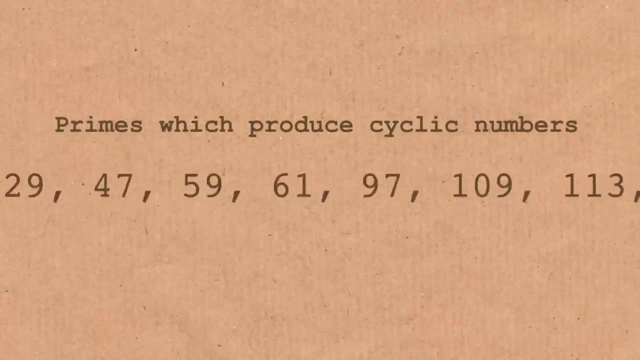 So the prime numbers that work, that give you, If you construct this, that will give you a cyclic number, are p, equals 7th, 7th, 17th, 18th, 17th, 19th, 23rd, 29th, the first few, there's more OK. 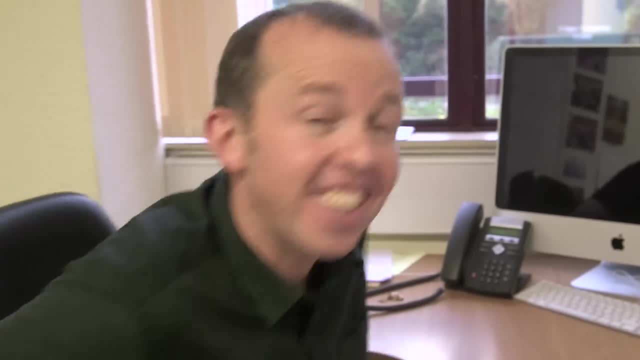 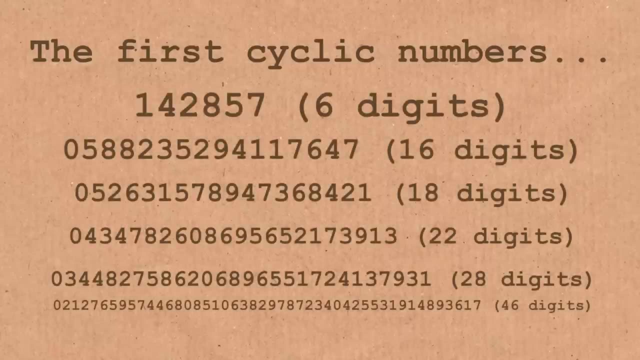 Are there an infinite number? There are an infinite number. yes, In fact, and this is one of these things that I just think number theorists. how do they dream up these things? We even know how many. what percentage of prime numbers give cyclic numbers. when you 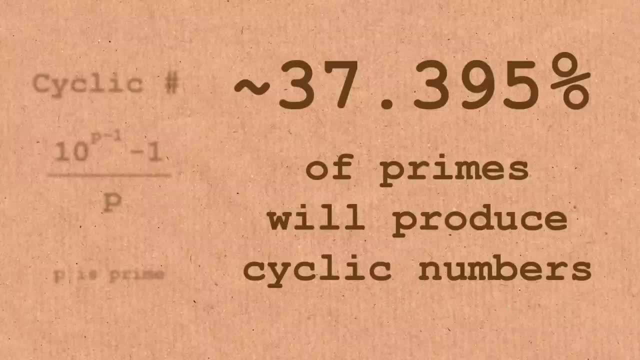 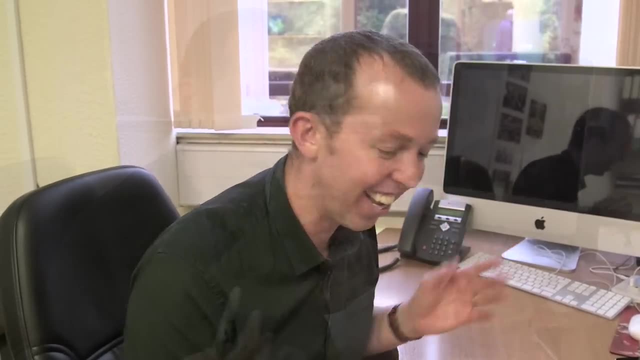 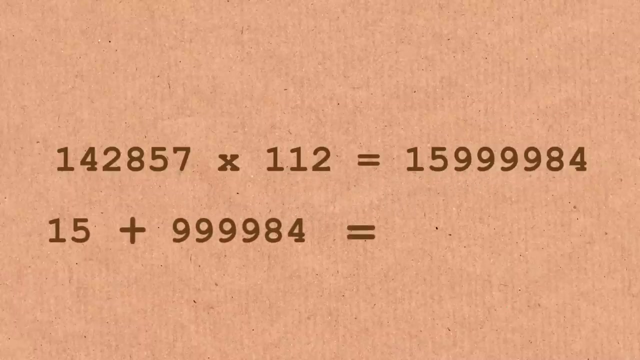 construct this- It's 37.395% roughly- of prime numbers- will give cyclic numbers. I mean why We saw how, if we multiply it by multiples of 7, and then we do our little construction that we discussed that, we get back all the 9s. OK, 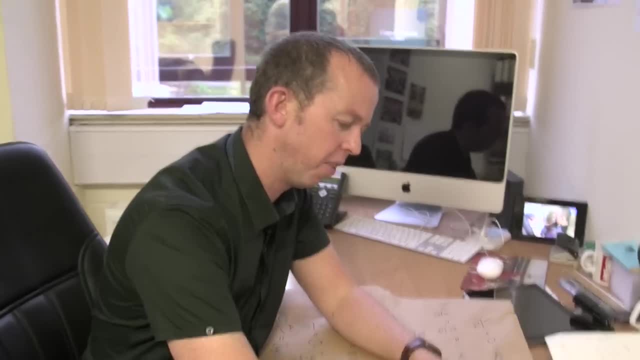 All the 9s appears everywhere in this. What else can you do? Let's look at it: 1, 4, 2, 8, 5, 7.. OK, let me take the first two numbers, Let me take the next two: 28.. 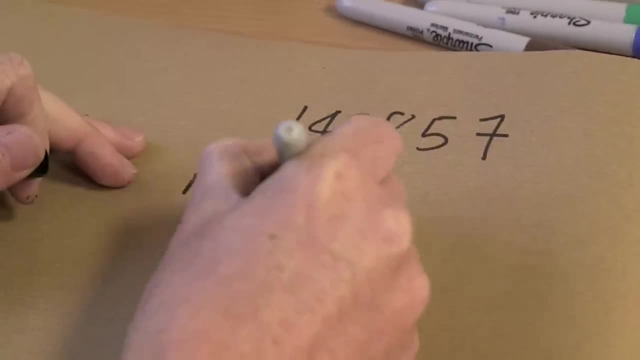 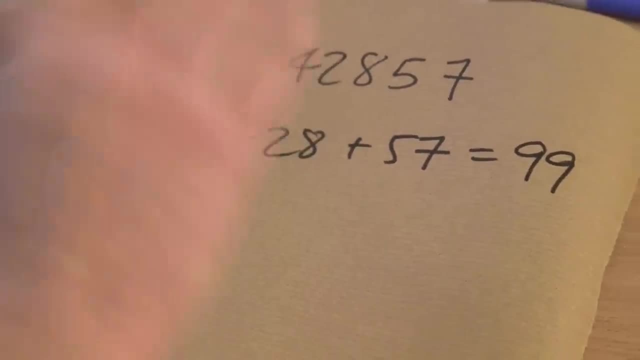 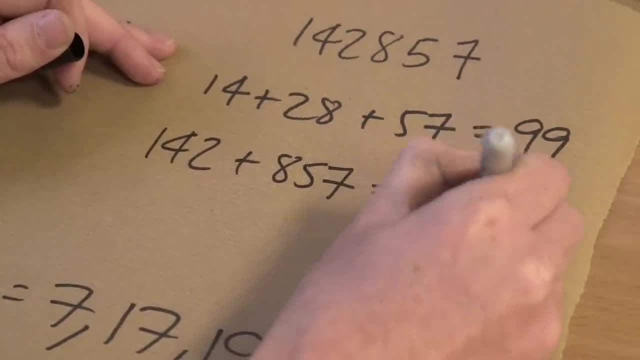 1,, 4,, 2,, plus 8,, 5,, 7.. I add them together. What do I get? 9,, 9,, 9.. Let me even do this. Let me do 4, right. 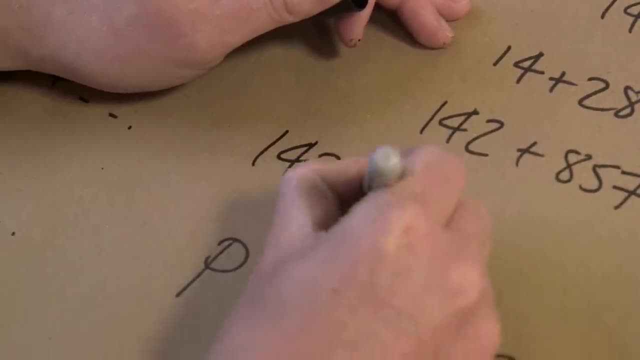 I get 1,, 4,, 2,, 8,, plus 5,, 7,, 1,, 4.. And I have to use every number the same number of times: 2,, 8,, 5,, 7.. 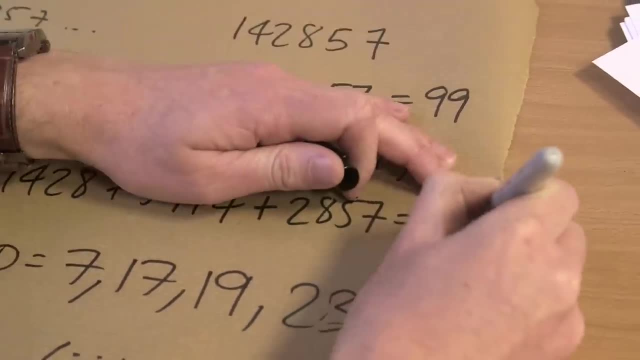 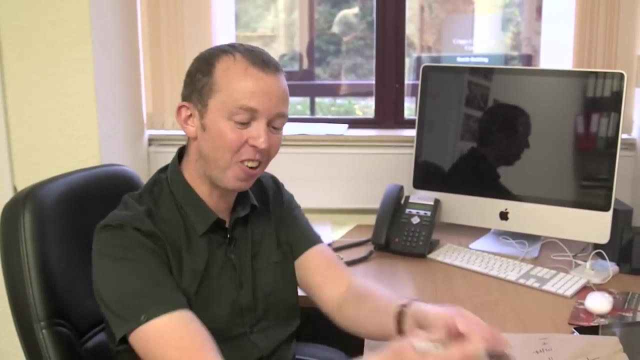 What's that? 9,, 9,, 9, 9.. That's amazing, It's amazing, It's amazing. I just love it. What is going on? It's all related, of course, to this very special property. 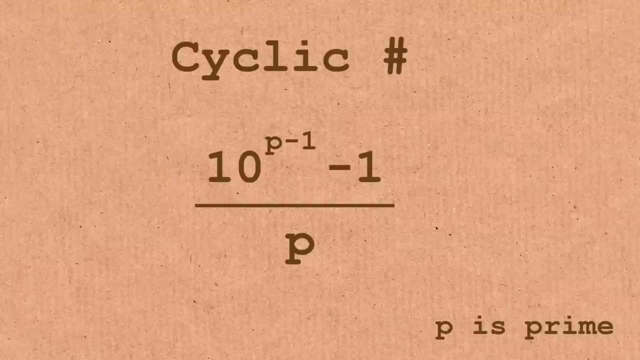 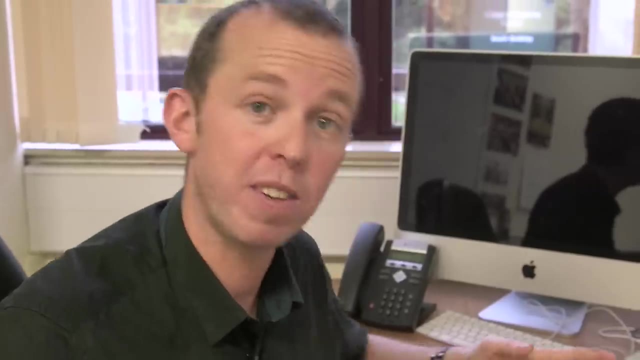 That it's basically. these numbers can be written as 10 to some power minus 1 divided by the prime number, But it's clearly just built in there And they all have this property. They'll all do this. You can also work in different bases. 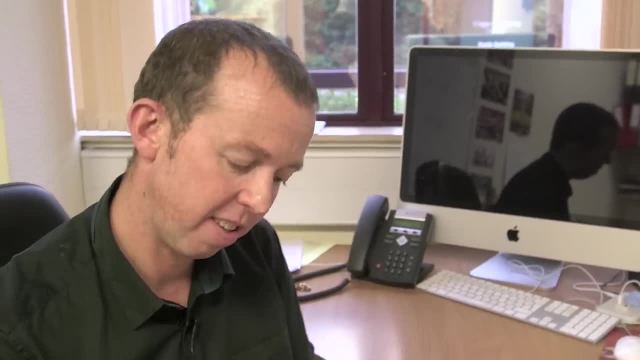 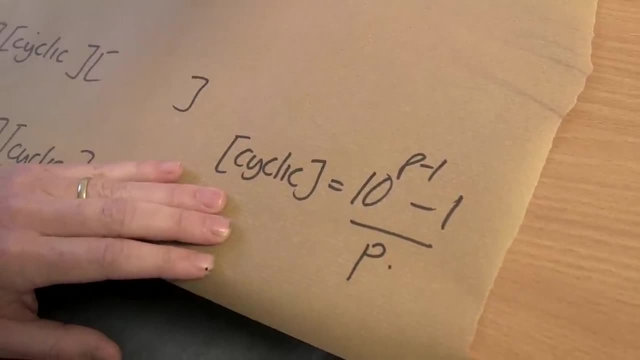 You can have cyclic numbers in different bases. What happens then is the cyclic numbers instead of being we're working in base 10, as we're familiar with, But you just change this number from 10.. And then you get the cyclic numbers again. 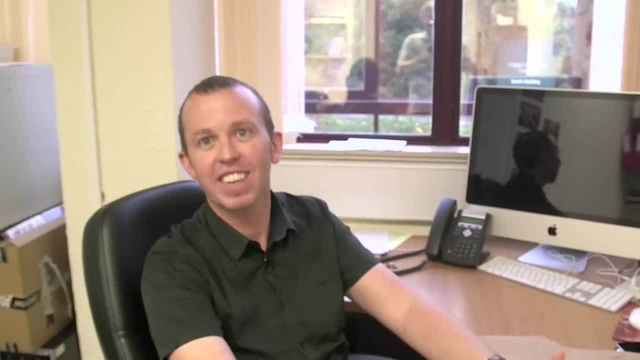 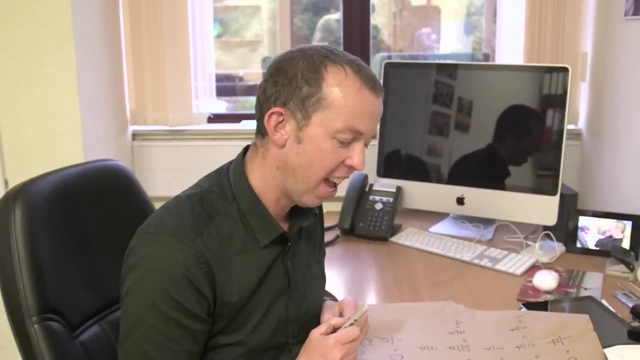 You can play the same games, But of course they're cyclic in that particular base And instead of getting all the 9s, you might get all the 3s or all the 4s, depending on whatever base you're in. 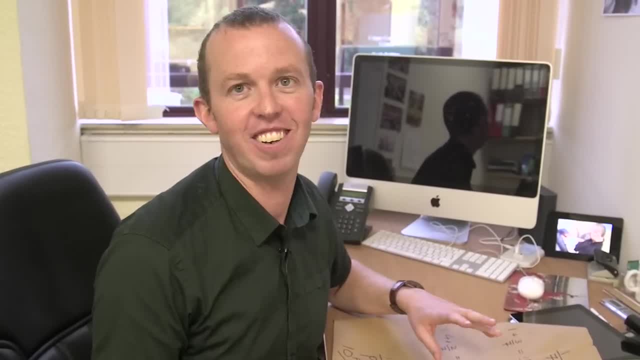 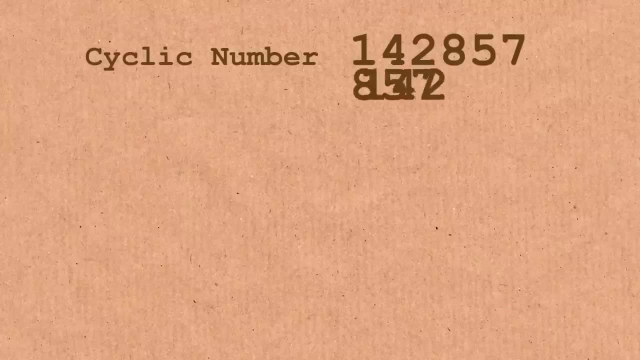 It's an amazing number. It doesn't even stop there. There's one more quirkiness that I've got to show you: 1, 4, 2, 8, 5, 7.. OK, Now we're going to take the first three numbers: 1, 4, 2,. 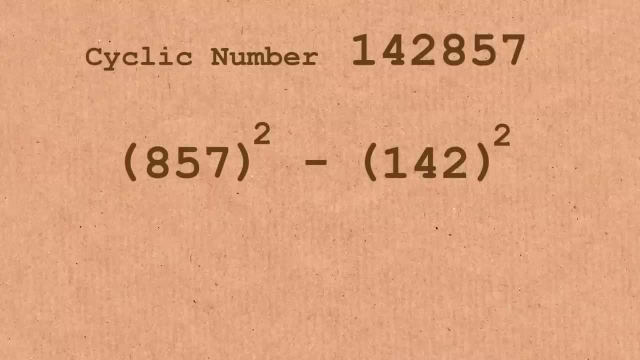 and square it to 8,, 5, 7. squared, What do we get? 7, 1,, 4,, 2,, 8, 5.. What's that? It's another permutation of our 1,, 4,, 2,, 8,, 5, 7.. 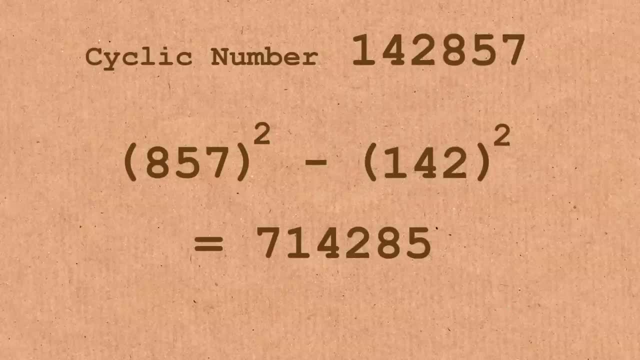 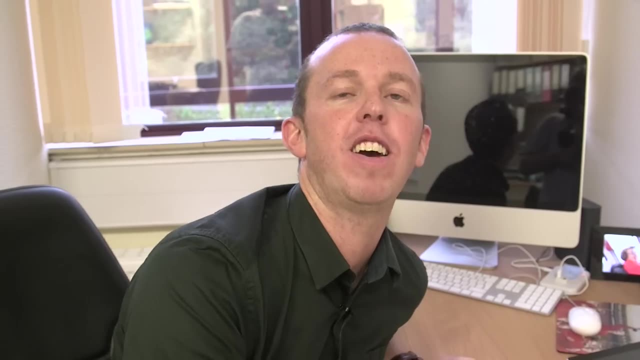 It's amazing And this number- actually we're not the only people to have noticed that this number has sort of quirky qualities. There's something called an Enneagram. Now this is some crazy Armenian spiritual leader from wartime called Gurdjieff. 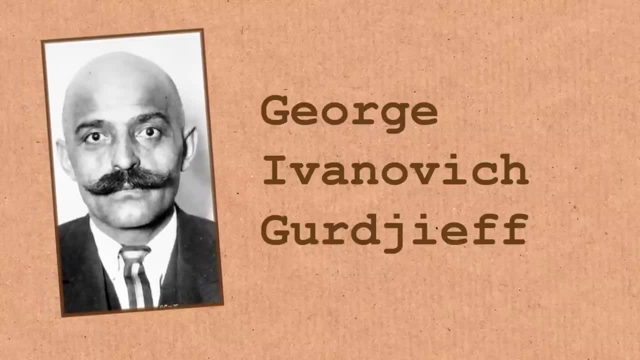 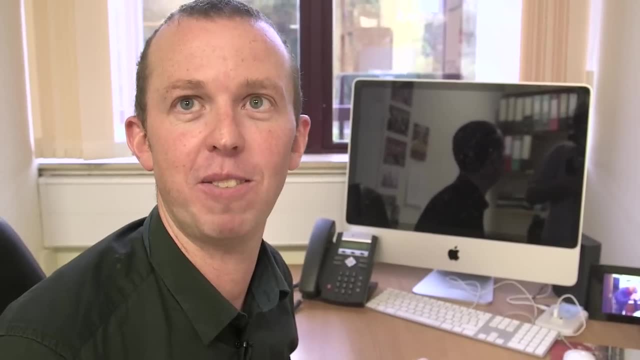 And he basically was able to explain everything in life and the cosmos through this number. It's total nonsense, The less said the better, But he did draw a nice pretty picture which I think we can draw, which sort of just gives us our last little thing to do.